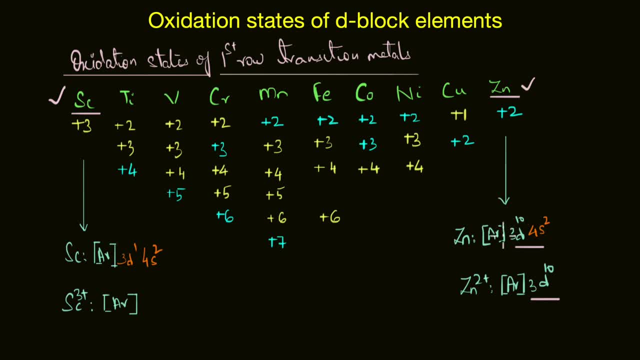 like in the case of zinc, is that you don't have enough orbitals available to share these d electrons with other elements. So once again that results in limited number of oxidation state. But if you compare these elements with those elements that lie towards the center, 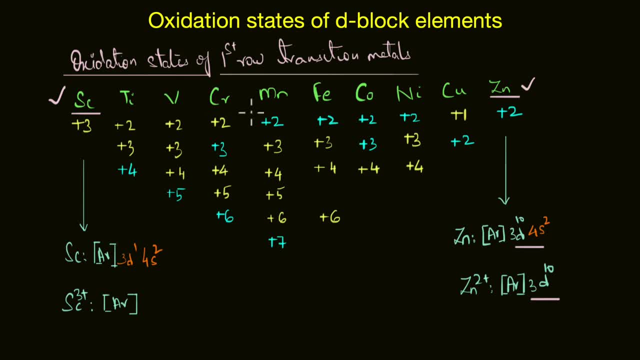 or the middle of the series, you can see that the ones at the middle exhibit maximum number of oxidation states. Look at manganese, for instance. Manganese shows oxidation states corresponding to the loss of electrons present in both 4s and 3d orbitals. That is, it ranges all the way from plus two to plus. 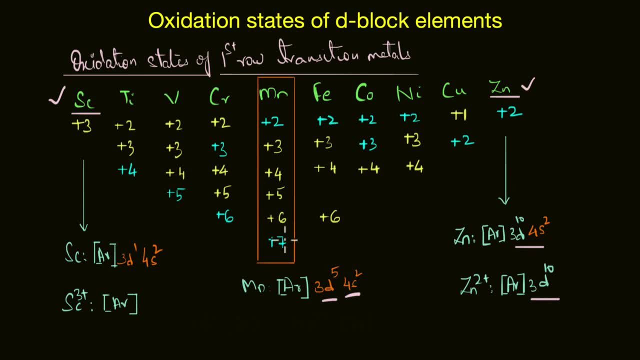 seven, Plus two when it loses two of the 4s electrons, and plus seven when it loses all of the 3d as well as 4s electrons. Now here again, as you can see, plus two and seven are the most stable oxidation states for manganese, because both of these state. result in stable electronic carved. Now here again, the flashingmap on the left is showing weak球 as compared to weak source filledhouse state. That is the least dangerous thing in comes before it getsết up, but this shows that mainly at low temperature. This is something 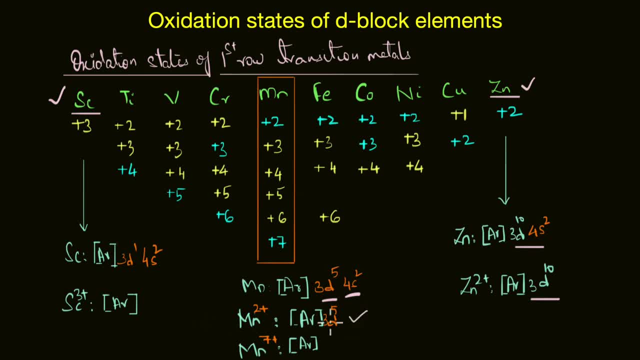 configurations. In plus 2 state you get half l d5 electronic configuration, and in plus 7 state you get noble gas configuration. Now, both of these states are most preferred because they result in stable states. Now, as we observe the oxidation states from scambium to manganese. another thing: 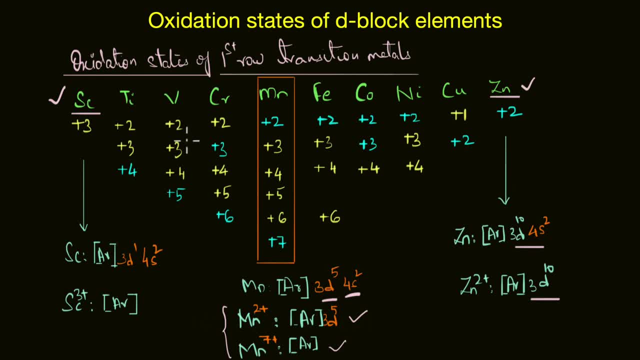 that we can see is that the maximum oxidation state corresponds to the sum of the electrons present in 3d and 4s orbitals. Like in the case of titanium, the outer electronic configuration is 3d2, 4s2 right, and that is why the maximum oxidation state corresponds to the sum of the 4s and 3d. 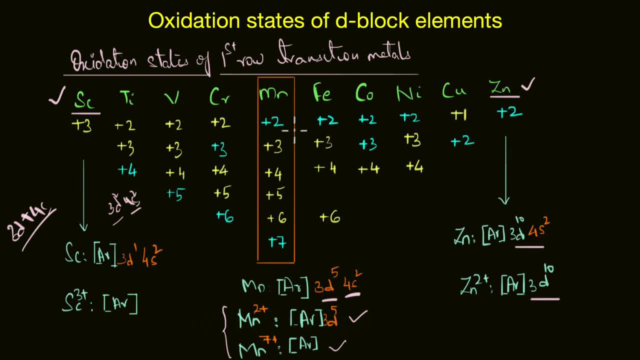 electrons. Similarly, in the case of vanadium, chromium and manganese, the highest oxidation state corresponds to the sum of the electrons present in both of these orbitals. However, from iron to zinc, if you see, we can notice a decrease in the stability of the higher oxidation state. In iron, the most stable state is plus 2 and 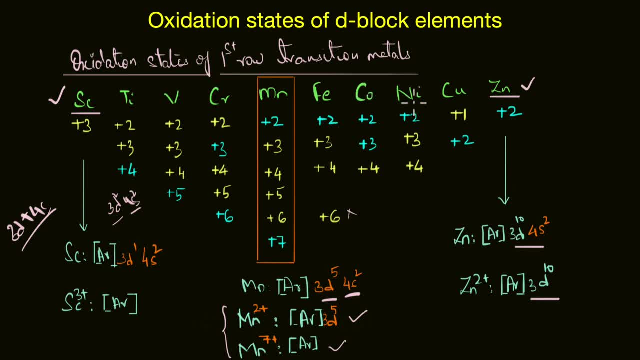 not plus 6.. Similarly, in cobalt and nickel, the most stable state is again plus 2 and not the maximum or highest oxidation state, which is plus 4.. Now, this decrease in stability of the higher oxidation states is because of the unavailability of empty d orbitals, or in other words, presence of 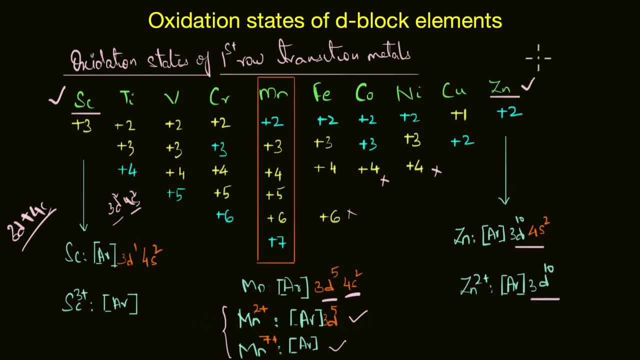 two many d electrons. This is why lower oxidation states get favored in the lower oxidation states, elements ranging from iron to zinc. now, these variable oxidation states are an important characteristic property of the d-block elements and, as we saw, this occurs due to the incomplete filling of the d orbitals. now another interesting 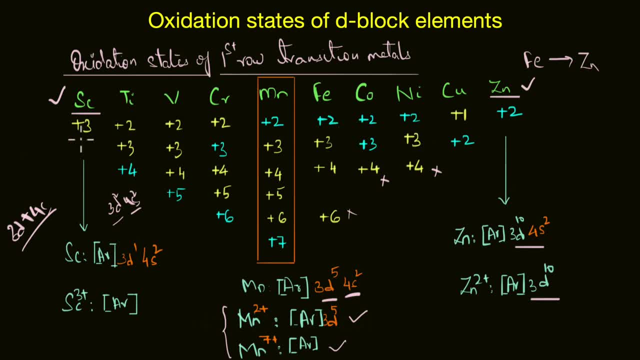 feature that might catch your attention is that the oxidation states in each of these elements differ by one unit: plus 2, plus 3 and plus 4 in titanium. in copper, plus 1 and plus 2. this is quite different from non transition elements, where the oxidation states usually differ by two units, for example, the 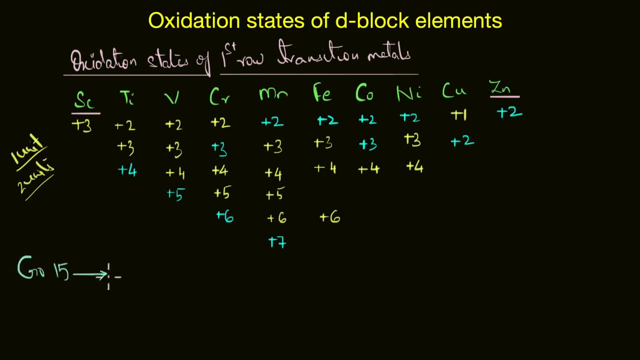 common oxidation states of group 15 are minus 3 plus 3 and plus 5. similarly, in group 16, the common oxidation states are plus 6 plus 4 plus 2 and minus 2, as you can see in non transition elements, like if you look at: 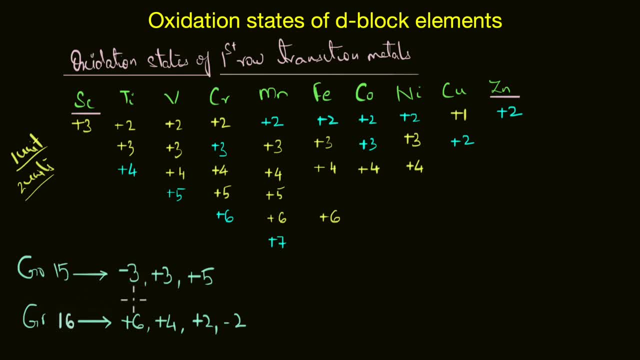 the p-block elements, the oxidation states of elements usually differ by two units, whereas in that of d-block elements or the transition elements, the oxidation states differ only by one unit. now, this is not the only difference between transition and non transition elements. a contrasting feature between d-block elements and p-block elements is the stability of the higher oxidation. 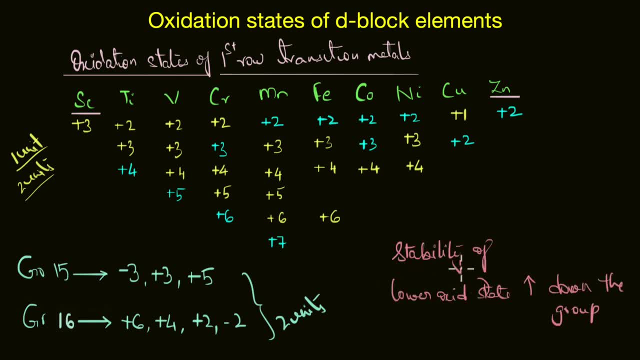 now, do you recall that in the p-block elements the lower oxidation state or the stability of the lower oxidation state increases as we go down the group? yes, it was due to a phenomenon called inert pair effect. so because of that, if you look at group 15, the lowest or the heaviest member, like bismuth, was more. 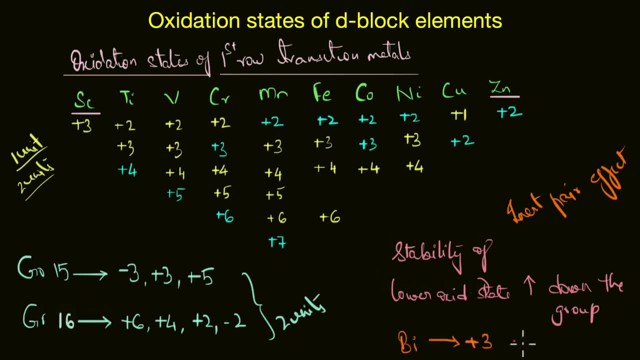 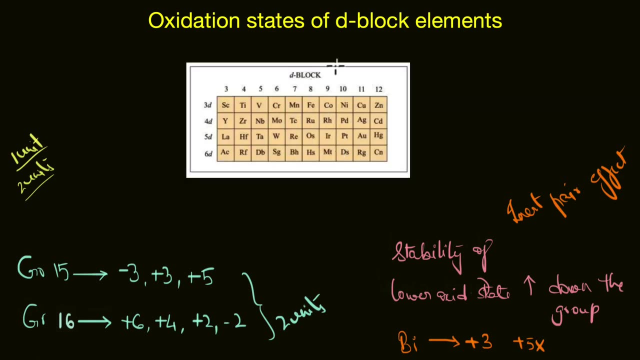 stable in plus 3 oxidation state and not in plus 5 oxidation state, which was a group oxidation state right. so here the lower oxidation states were more stable or more preferred. however, in d-block elements it was found that as we go down the series, higher oxidation states.